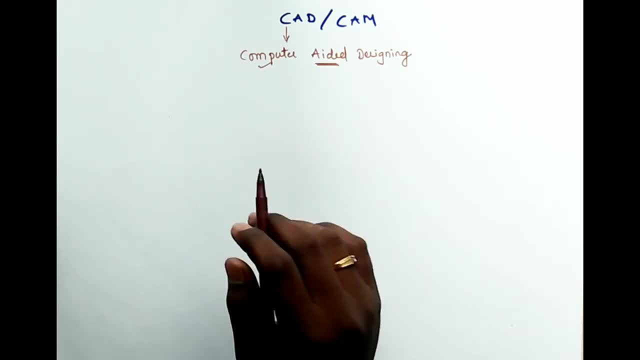 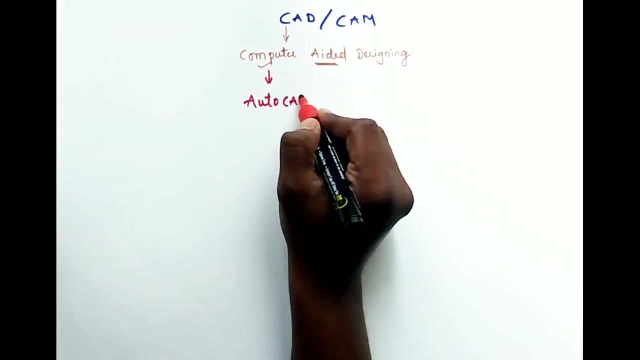 Here. one more thing. one more important thing to be noted is we are going to use different types of softwares. when it comes to computer aided designing, For example, the basic software we are going to use here is AutoCAD, The basic tool. what you call AutoCAD is actually a. 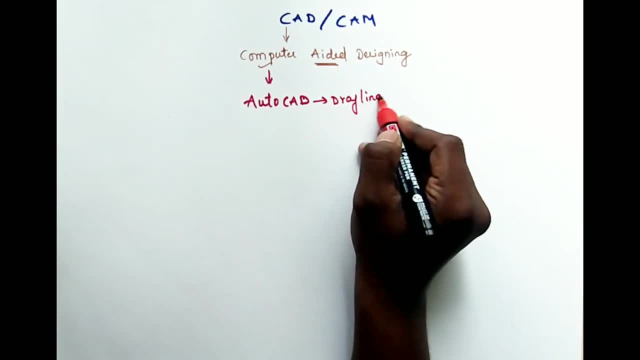 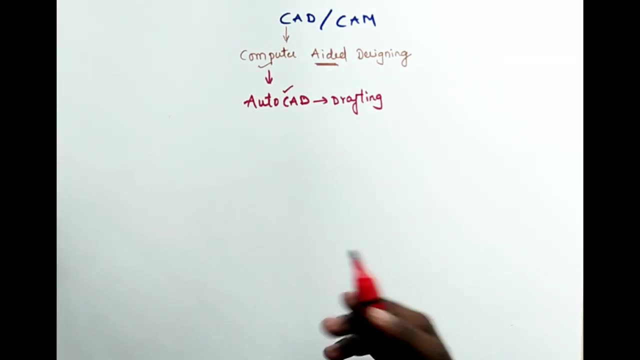 drafting tool. Drafting tool. Drafting tool. Ok, You can avoid the traditional way of drawing by using this particular AutoCAD. Traditional way means we are trying to use a drawing sheet, followed by a drafter and all the drawing instruments. The person who is going to draw is called as a draftsman. Same work can be. 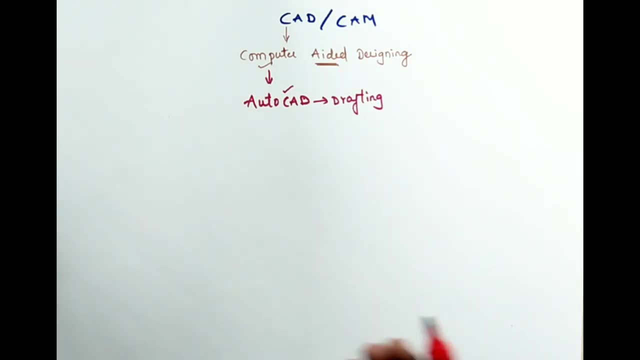 performed by using AutoCAD, Ok, where you can avoid the drafter, drawing table, drawing sheet and all the drawing instruments. Only a simple software will help you to draw all your layers, Ok, or whatever the sketch you want to make on the sheet of paper. okay, that can be. 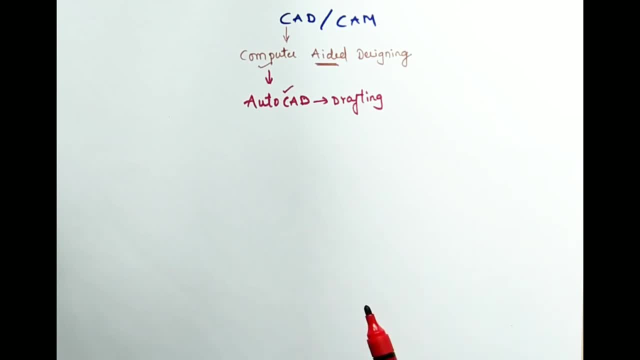 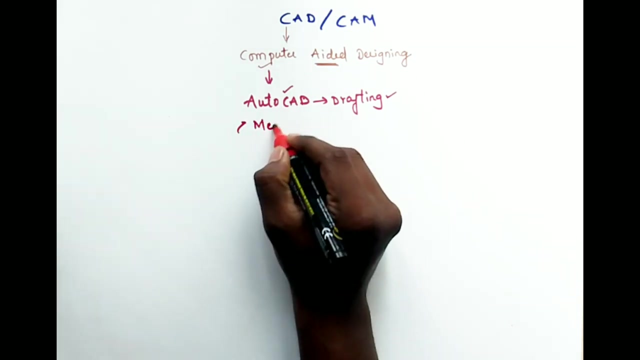 done using a software and the same can be taken as a hard copy with the help of printers. okay, now here, if you talk about AutoCAD, how to care is all about drafting. okay, any sketch can be drawn, any layout can be drawn. okay, this is used in general. if you talk about mechanicals, mechanical students or 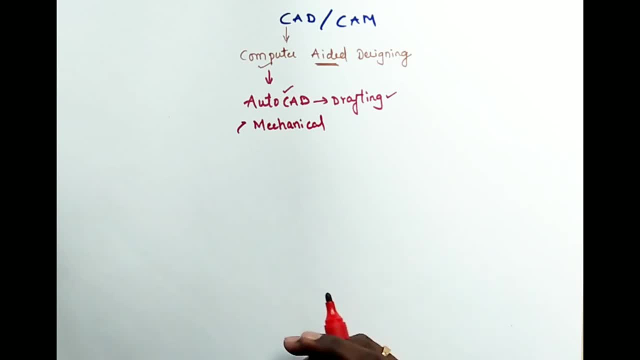 mechanical field, most of the mechanical related industries. they use AutoCAD, okay, and other. next is civil in the construction area to draw the layout of a building, to show the proposal to the municipality for an approval. civil people will also use in constructions of a building, of a dam, okay. 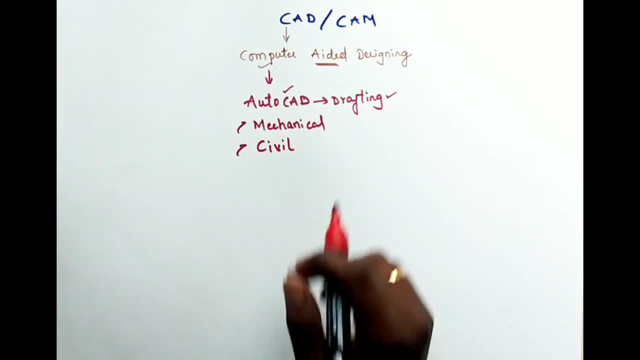 any other construction they'll use it in general. okay, other than these two. broadly, these two people like mechanicals and civils. they use AutoCAD software. okay, other than this. the same software can be used in electronics and electricals and many other fields also. okay, but mostly the percent is bit higher. 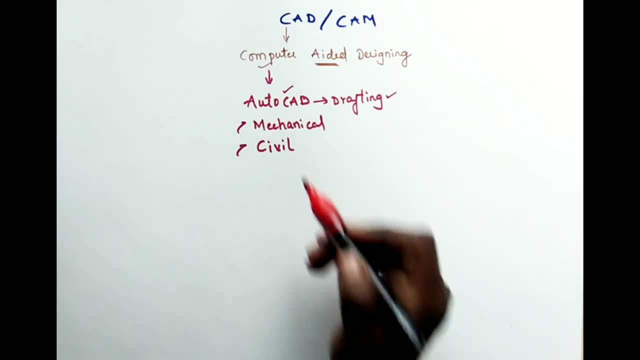 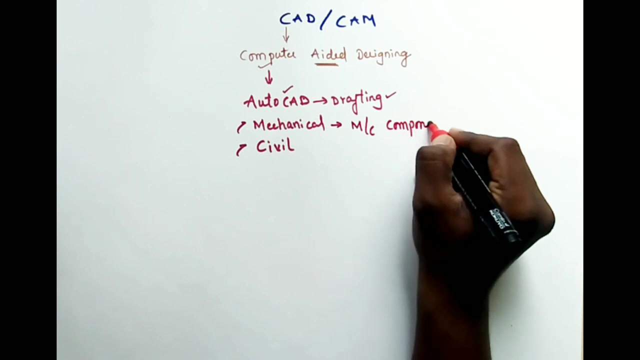 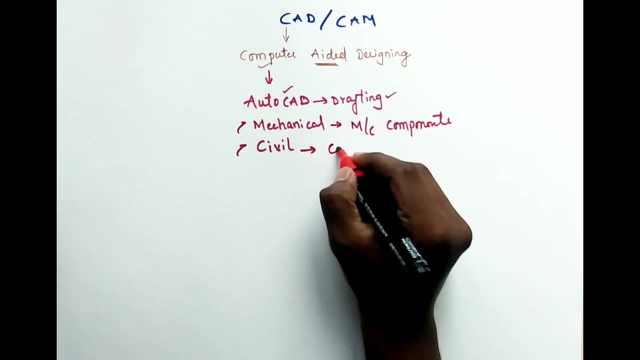 okay, but mostly the percent is bit higher when it comes to electronics and electronic engineering. mechanicals and civils: okay, these mechanical people, they'll try to use it to design, to draft what you call a machine components, to draft machine components, okay. and civil in construction, in construction, okay. 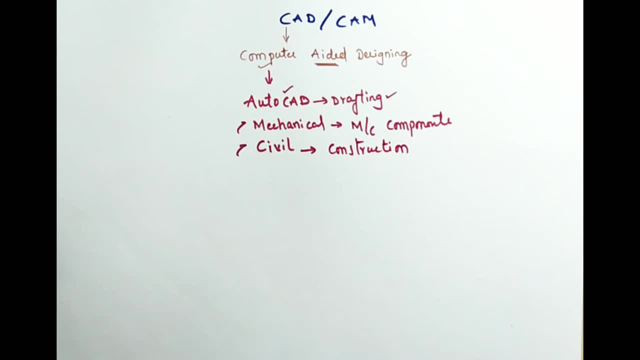 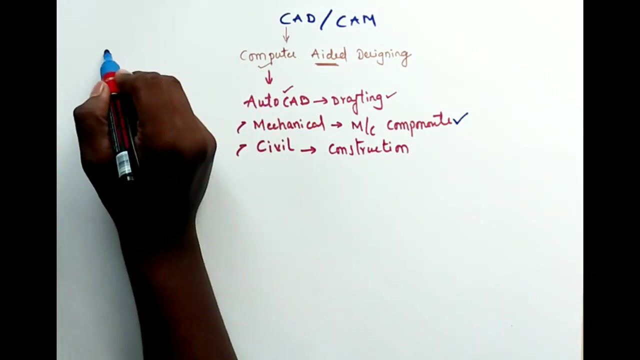 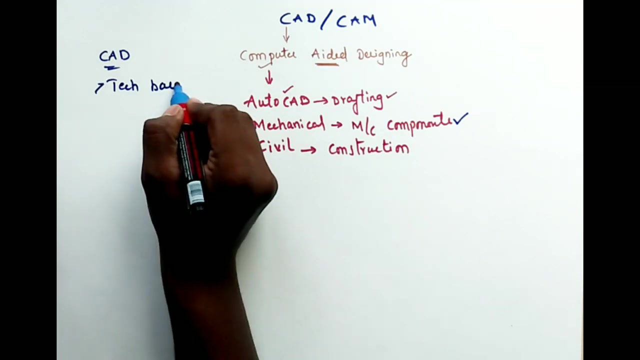 and today we'll try to limit our discussion to mechanical engineering. we'll limit our discussion till here. okay, how does it help? it is a technology base, okay, CAD? what is CAD? CAD is a completely technology based, what you call technology base for the computer integrated factory. okay, technology base for computer. 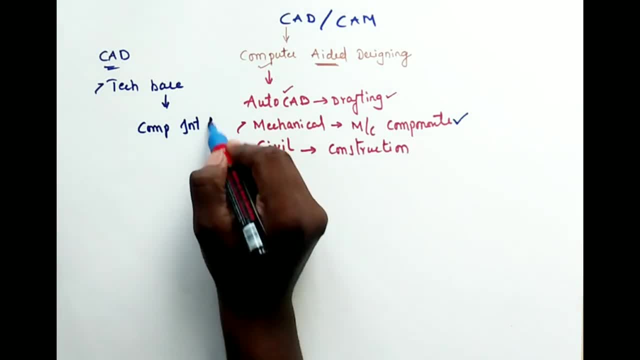 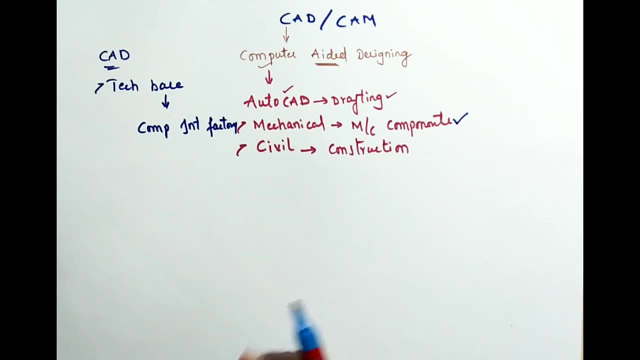 integrated factory. okay. so if you want to draw anything, if you want to make a layout or if you want to transform that into a 3d model, everything is possible in this particular software. okay, for whatever the future, upcoming future, technology will keep on improve or keep on increase. it all depends on the 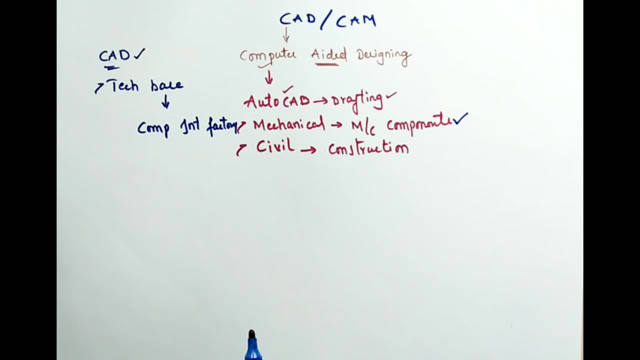 advancement of the technology. okay, computer aided designing can be defined as use of computer system to assist. okay, now, this computer system will help you to assist in creation. creation means it all depends on every individual person. it's his perception. okay, now, for example, creative mind will help you to get new thoughts, will help you to get new things in the society. 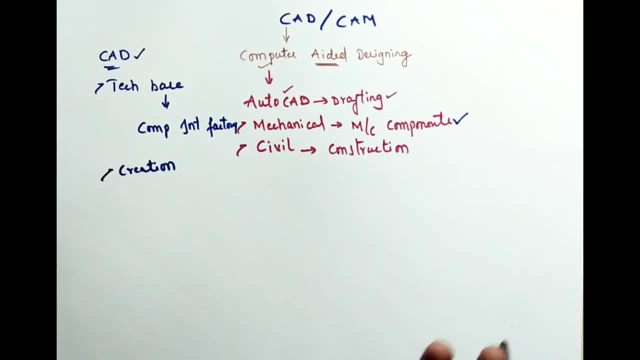 okay, it all depends whether you belong to an automobile industry or an aerospace industry, or maybe you belong to some garment industry or a factory. okay now, autocad is used in every industry, irrespective of its. i know it, doesn't? it just not belongs to mechanicals or civils. it has been using from past many years in many other industries. okay, creative. 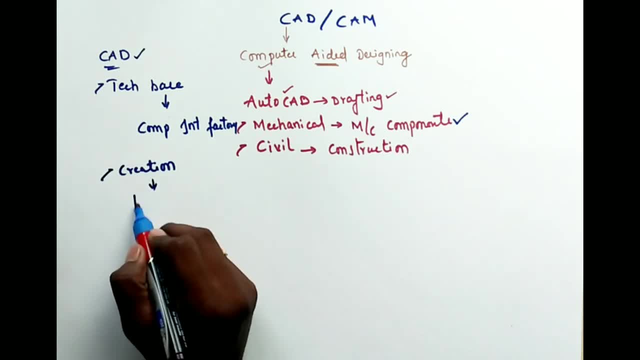 mindset is more important. uh, with this you will get a thought. you'll get a thought to make something new in the society. okay, maybe it all depends on automobile, or whether it is an aerospace industry or some other x industry. okay, so creation is one and one more if i talk about is modification. 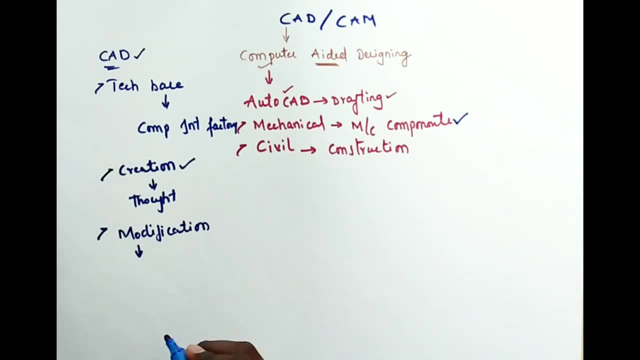 now here the. if you talk about modification, modification is all about, uh, already existing component. if something is existing already, if you want to make some changes to improve its efficiency or to improve the aesthetic appearance of the model, that can be done okay, appearance okay. or else, uh, to improve efficiency. 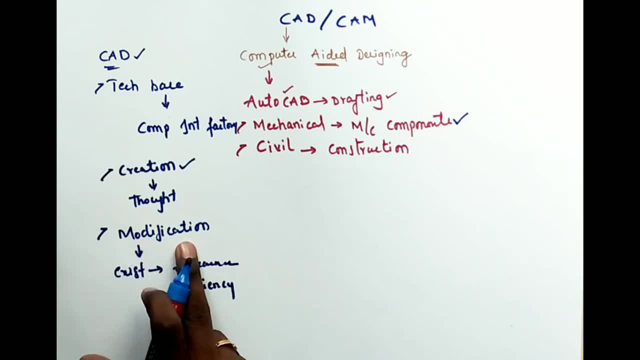 or else any other thing. if you uh just with the help of modification, if you can do the cost cutting also, it will also help uh productivity. okay, so many other modifications other than this cad also help you in analyzing, analyzing. okay, analysis can also be done, analyzing, or you can call it as optimizing. 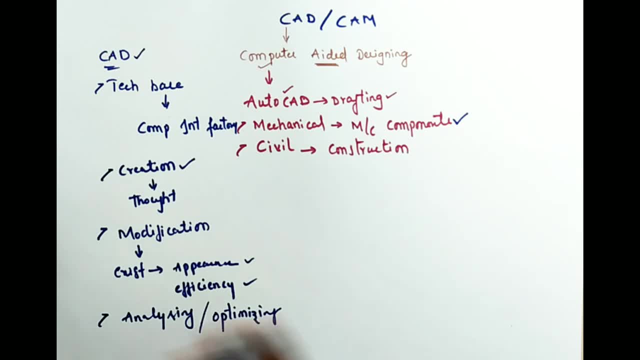 optimizing of a model or any other creation. okay, now, if you talk about analyzing, analyzing is all about. if you talk about the mechanical point of view, mechanical point of view, analyzing all about. once you have modeled, you have created a component that need to be analyzed for whether the same component is worth full or not. will it take the 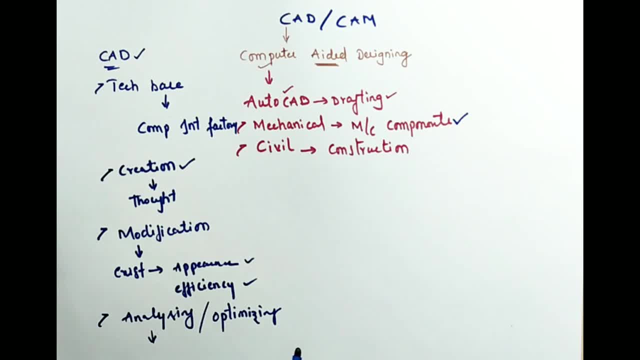 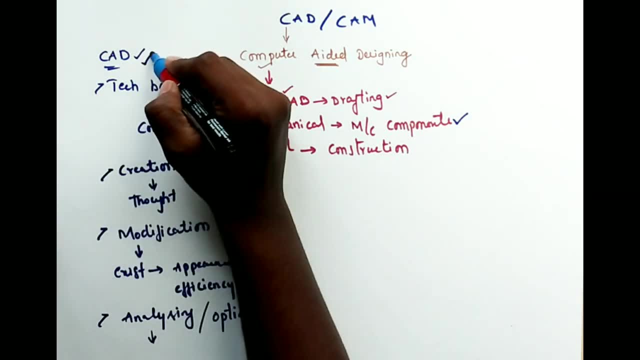 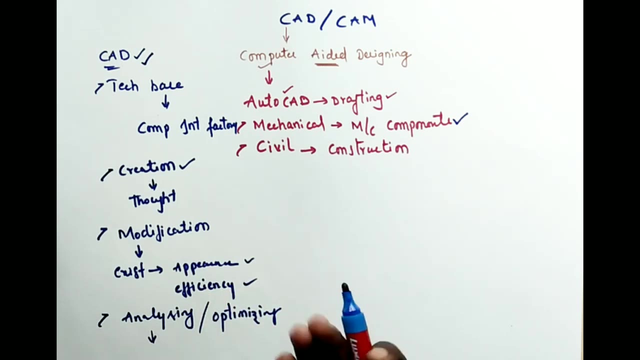 loading conditions required for so and so. environment or not, that has to be decided before manufacturing. okay, uh, we are talking about cad system. we are talking about cad system. we are not into manufacturing, we are into designing. we are talking about manufacturing. we are talking about where you can make conceptual drawings. you can transform that, your 3d model. 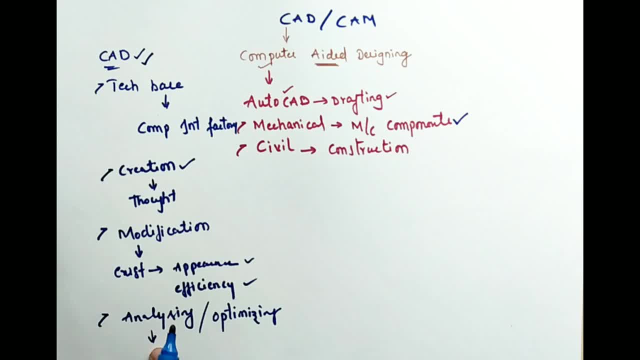 then you need to analyze the model here itself. okay, analysis can be done, for example, structural. structural analysis, okay. or thermal analysis, or fluent, it all depends. all these belongs to mechanicals, okay, okay, fine, for example, I have, I have created a component. I have developed a component. I have developed a. 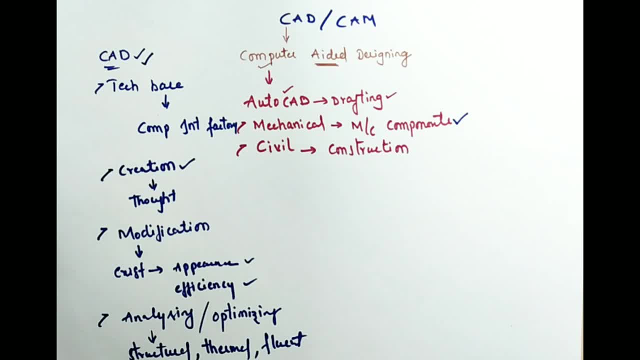 hexagonal nut and a bolt. I need to check whether it will take that much torque or not, that much force or not, before manufacturing. only I'll try to analyze by doing some structure analysis, by applying some constraints, boundary conditions, then followed by the loading conditions. then I could analyze myself. 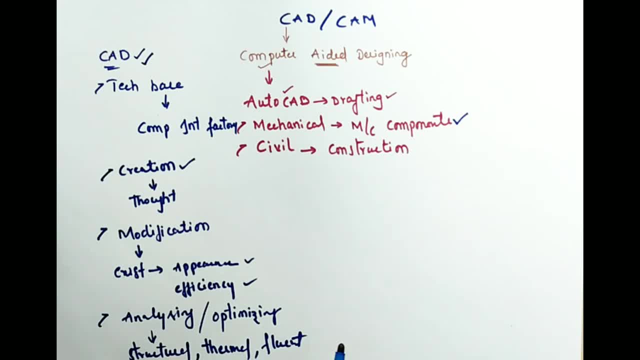 that yes, fine, so and so X component is feasible, so to so and so environment. once it is done, then I'll go for manufacturing. okay, without doing an analysis part. if you go for manufacturing, there will be a wastage of many things like, for example, if you talk about, there is a little bit. 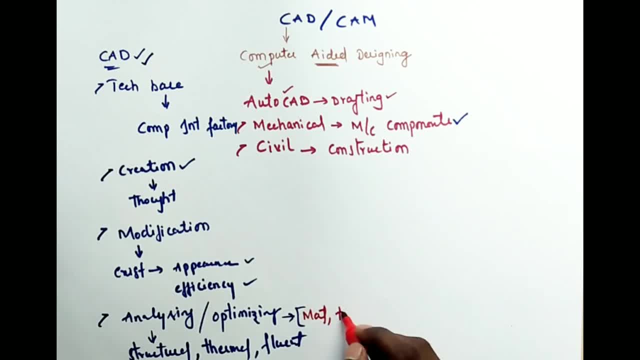 maize stage of material. time, money, manpower, many other things, okay for science, a purpose. you may procure machinery, you may procure tools, you may procure many other required new invented tools or a material, different types of materials. So once, without analysis, if you try to go for production, if you try to go for production, 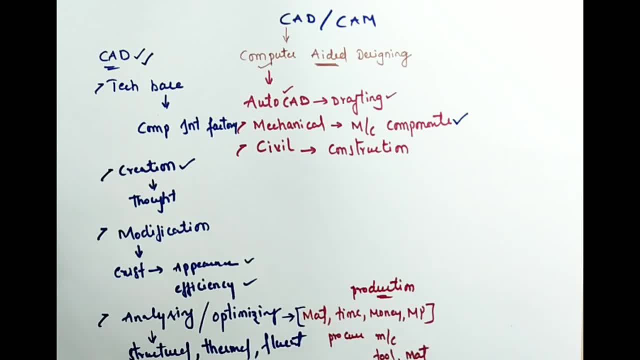 there will be a wastage of these many things. Time is a very big, important thing in case of productivity And fixtures, jigs and fixtures also- you try to purchase from the vendor. So all these are wasteful job If you don't plan your thing. 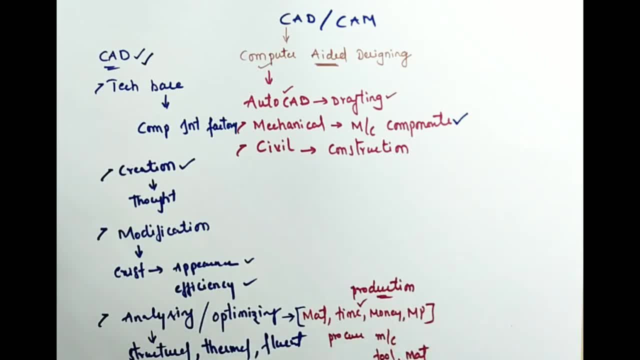 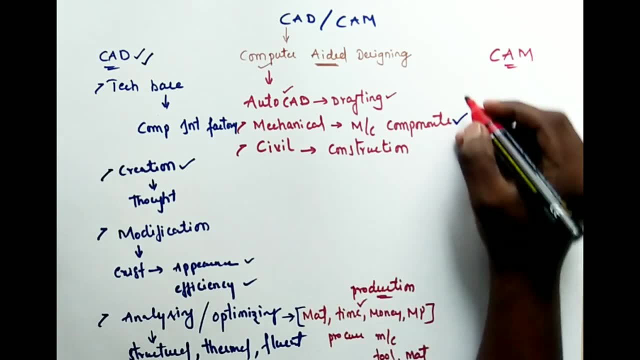 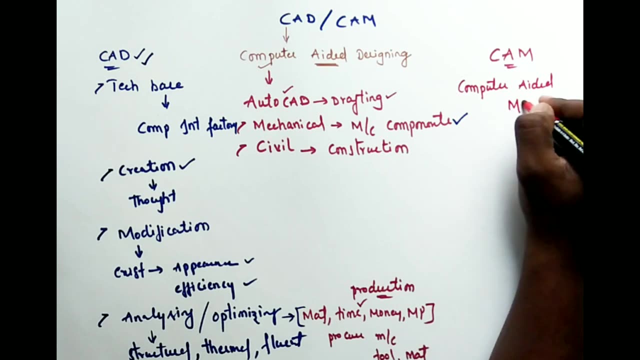 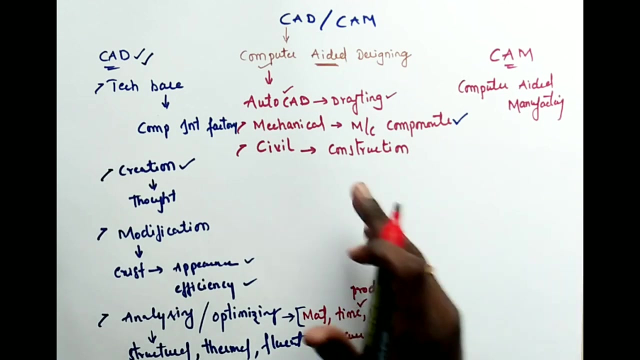 If you don't plan your things properly before going for manufacturing. before now I'll talk about manufacturing, computer aided manufacturing. The full form is computer aided manufacturing. Computer aided manufacturing- where we'll reach to this computer aided manufacturing once you finish the manufacturing. 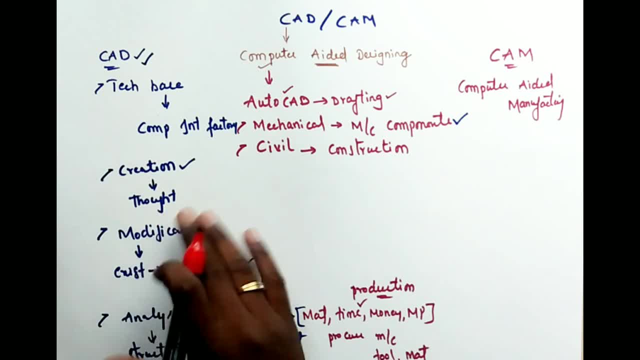 Then we'll go on to the manufacturing process, which is most important thing to be done, Without doing all the stuff. if you reach the manufacturing or a production process, it is again a wasteful job. Okay, Now, this is a very important thing to be done because if you don't do all the stuff, 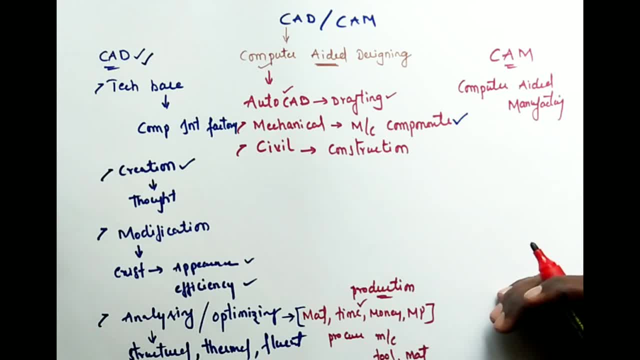 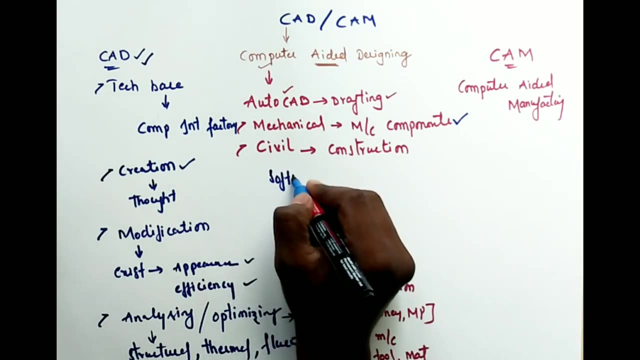 you will not be able to do the manufacturing process. you will not be able to do the manufacturing process. Okay, So this CAD software. if you talk about software or a hardware now, for example, if you talk about the software other than AutoCAD, other than this particular AutoCAD, you find many. 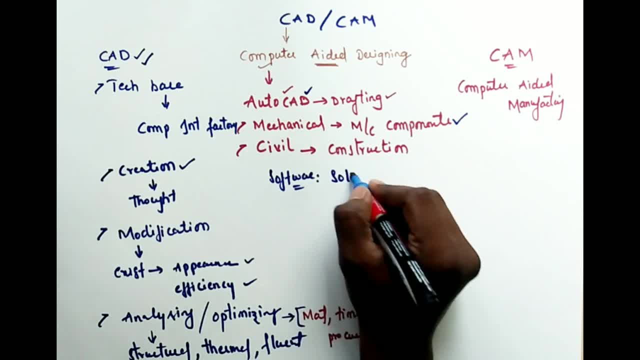 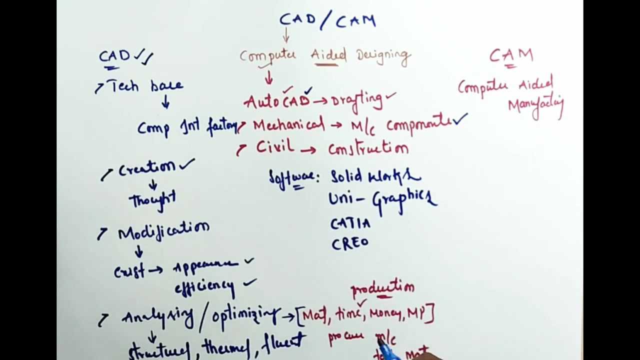 other softwares in the market, like SolidWorks- SolidWorks, okay. UniGraphics, Okay, Okay. And thi Catia, Catia, Creo. likewise, you have many other softwares available in the market. Okay. So by using any of the softwares, model can be created, but why we are using these many? 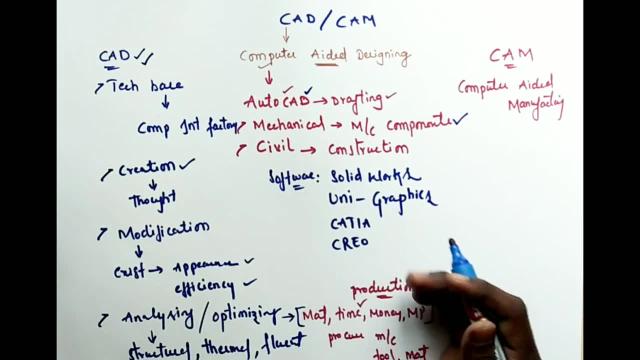 number of softwares, when the same model can be created in any of the softwares. So it all depends on the flexibility, so it all depends on the user friendliness, Okay, of so and so x softwares, and it also depends on the industry which they are using it, whether it 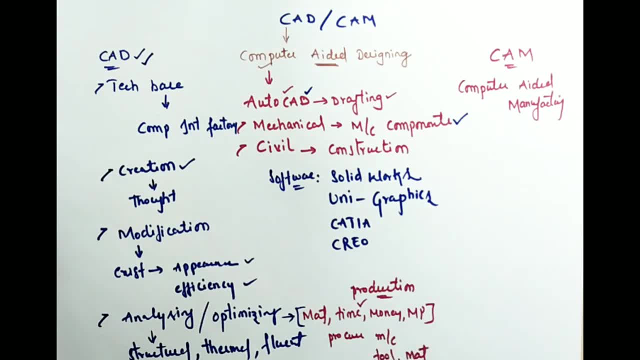 is a small scale industry or a large scale industry. okay, if you consider uni graphics, it costs more. if you consider the commercial uni graphics software, the cost is very much higher. okay, if you consider again katia, the or a creo, the cost is very much higher. okay, it all depends. 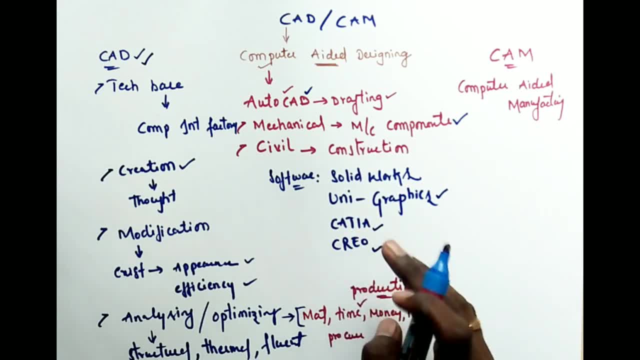 and. but if you try to purchase this, if you want to work over it, it is a very much user friendly and very much helpful to create your model or optimize your model. it will help you in many cases. the accuracy will be more and there is a proper precision of so and so component created and 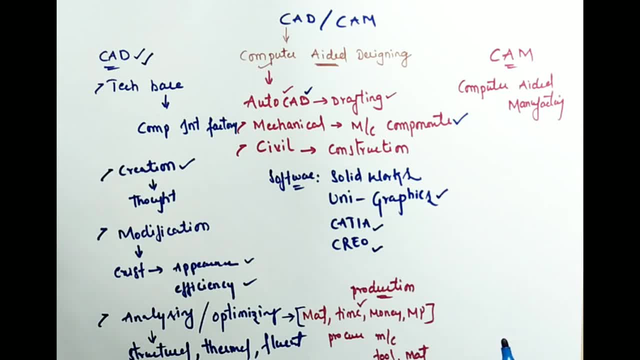 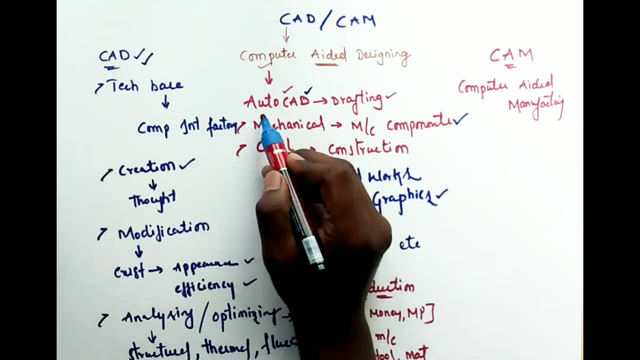 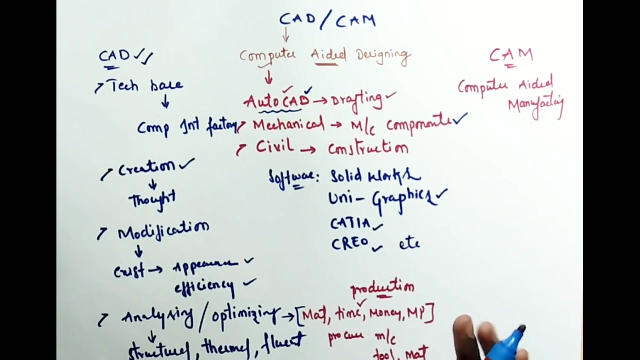 documentation will be, uh, at high end. okay, these are all very more. many, many more advantages are there by using these particular softwares: the video linkfill, the code where you will be able to buy a set of software of any andere 쪽��. this software is quite pinpoint, which then it will give you a checklist of Algorithm. 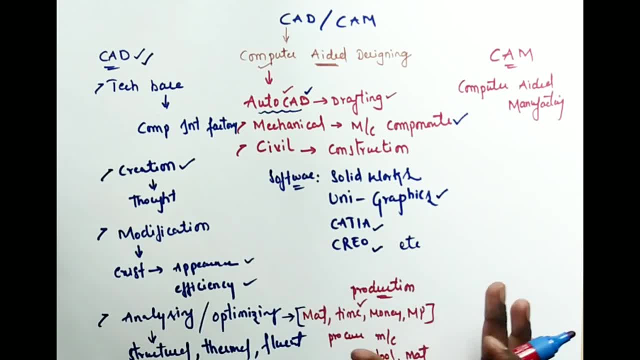 Attribution list as well. so, basically, the seocat software is gonna give you all those criteria and okay, so so we're gonna talk more next and then we're going to go to our another video, which is an snack chapter, So it will give youему a little bit about the sophisticated software. these are the warning. 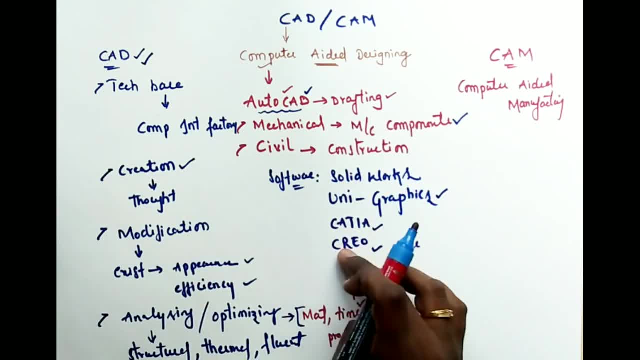 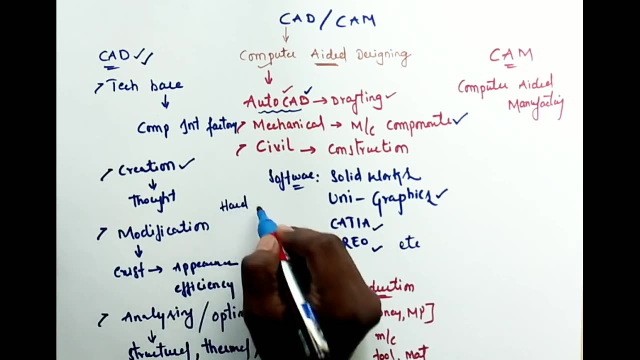 about wireframe modeling. okay, so other software are also existing in the market, can be used once you're done with your thing. if you talk about cad hardware also typically includes computer, simply okay. if you talk about cad hardware, cad hardware- this includes, as you all very much familiar with, a computer. 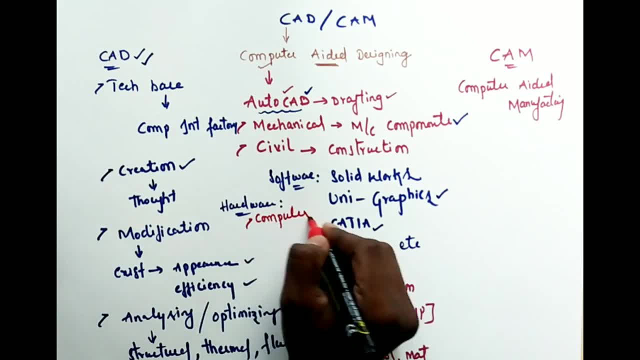 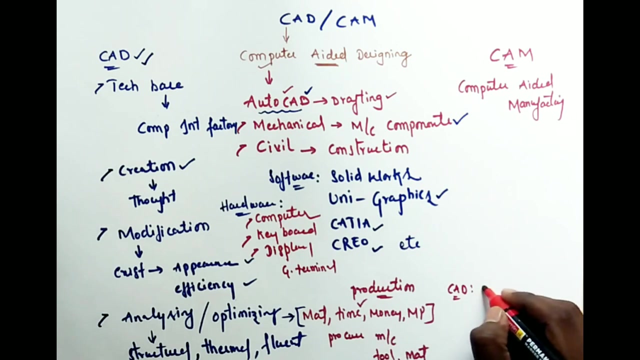 this includes a computer, a keyboard, a display terminal. okay, a keyboard, i'm not going into much deeper- two or more, one or more display terminals- graphic terminals may be graphic terminals to have a very good visual effect. okay, Now, CAD is what? Again, if you conclude, CAD is a designing tool, CAD is what? Designing? Use it for a purpose called designing and drafting. Designing and drafting, Okay, You can do, synthesize the model, You can analyze the model, You can document the model also. 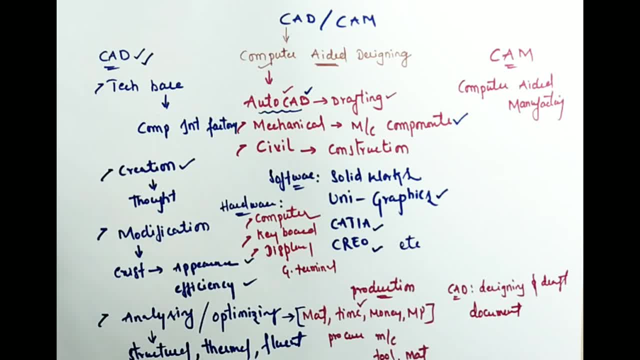 Document the model also. Whatever the tasks you have performed can be documented for the further process of CAM. Okay, You can do process planning also in case of CAM system, That can be done by using this particular documentation, which is very much important again. 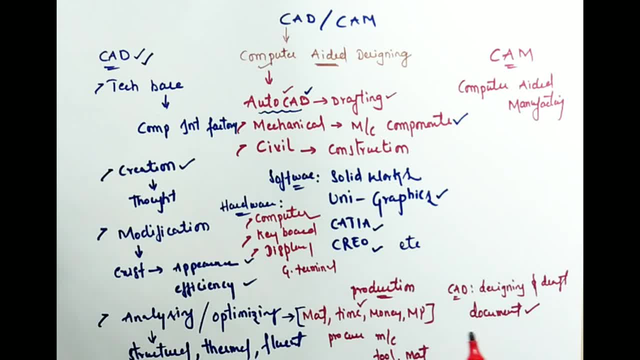 Okay, These are all the things required. CAD software, again, if you talk about only CAD software, consists of computerized software. Computer programs to implement computer graphics of system- Okay. Plus application programs of facilitating the engineering functions of. Okay, These are all possible with this particular software. Now, if you talk about CAM system, which is computer aided manufacturing, If you talk about the manufacturing here again, without much involvement of a human, you can do things with the help of software. 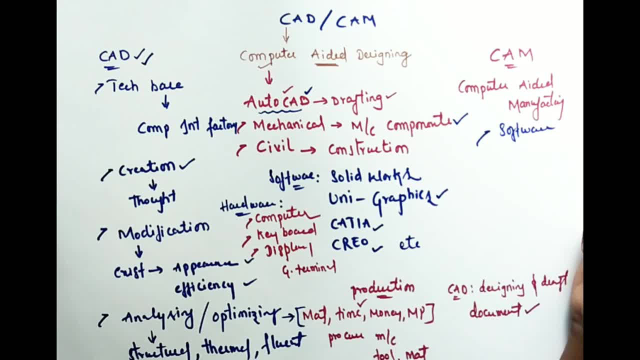 Okay, There are CAM softwares available in the market which will help you to manufacture, which will help you to write a program based on G and M codes. Okay, To manufacture So and so, X component. Computer aided manufacturing. Okay, In a similar fashion, you have computer aided engineering. Okay, Model generator, CAD, CAM. If you talk about 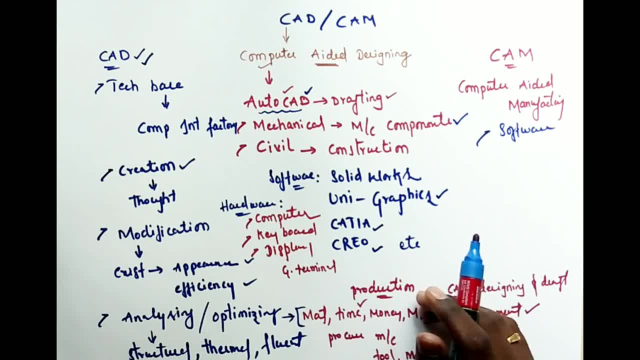 Only CAD system. you can create Prototypes. you can create a finished models also. Prototypes can also be prepared. You can have a visual effect before manufacturing your component with the help of 3D printing. with the help of 3D printing, You can visualize a 3D model how it is going to be after manufacturing- in the initial level only before manufacturing- which will help you to have a visual effect of a component and if some changes. 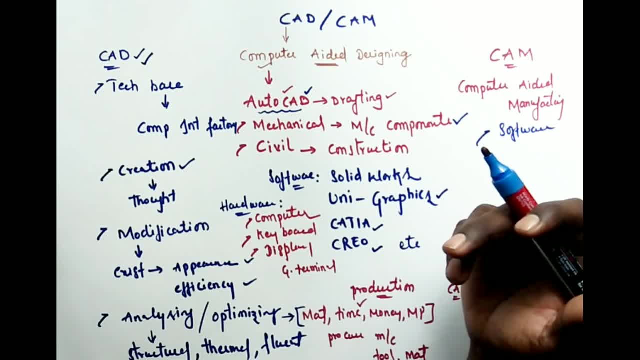 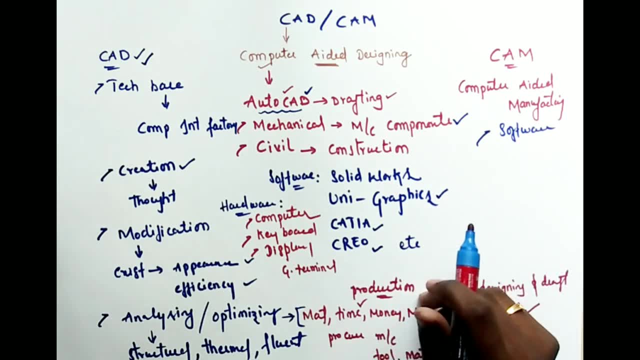 required. that can be done by using again a cad model or programming can be changed to reach your destiny. then once it is done, once everything is okay, then you can go for manufacturing. okay, that is possible. and to have a tool path. to see the tool path, whether the program written is right. 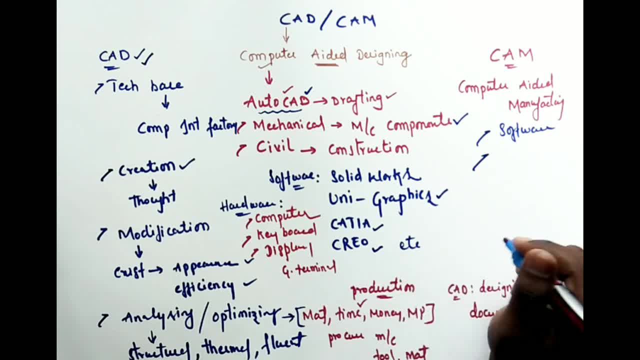 or wrong. to have a proper judgment, you have many other software developed in the market. the basic one if you talk about is you have a software called edgecam. edgecam which will help you to show the tool path and if everything is everything goes wrong, you can take that same program to the.